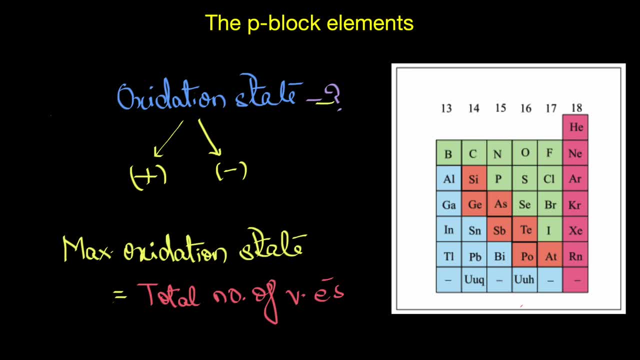 Well, you see, the maximum oxidation state an element can show depends on the total number of valence electrons. Now, in the case of p-block elements, the total valence electrons is nothing but the sum of the s and p electrons, Right, For example, if you go back to the group 13 elements, 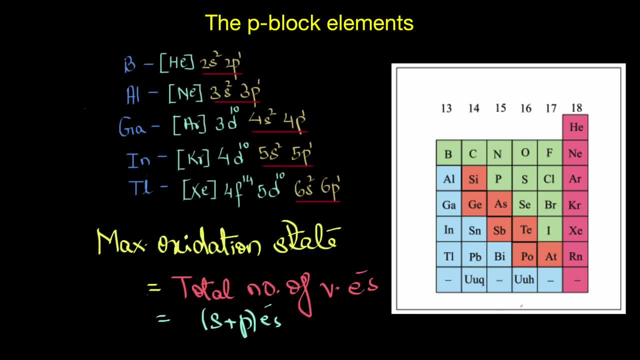 again, you will see that the maximum oxidation state any element in this particular group can show is a total number of valence electrons which is nothing but the sum of the s and p electrons. that's again three. that means these elements will have to lose three electrons in order to attain a stable 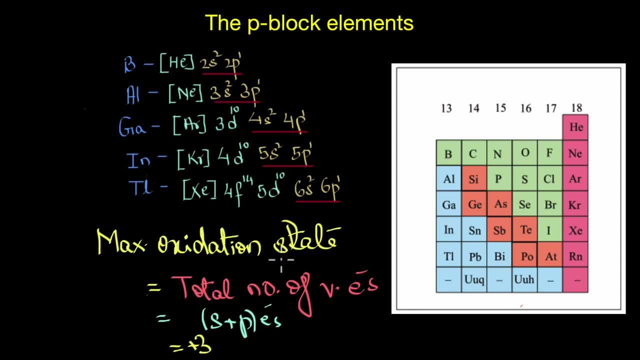 electronic configuration. now remember, folks, when we say lose or gain electrons to attain stability, this is purely based on how oxidation state is defined. as we know, it is a hypothetical charge that we assign to an atom, assuming that the atom forms only ionic bonds. now, this is important. 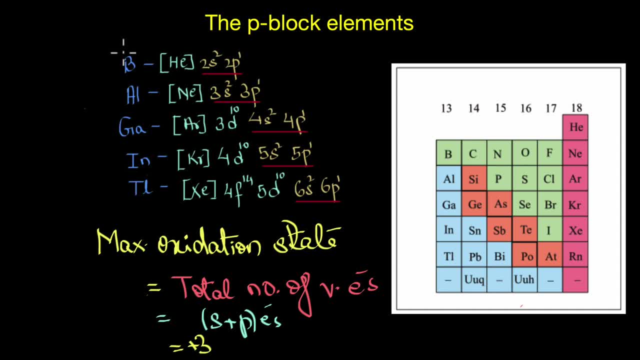 because you see, boron, just as many other elements in the p block, does not lose electrons. you know it does not lose three electrons to form b3 plus ions. it actually shares these electrons but still, while assigning an oxidation state, we assume that the bonds that boron 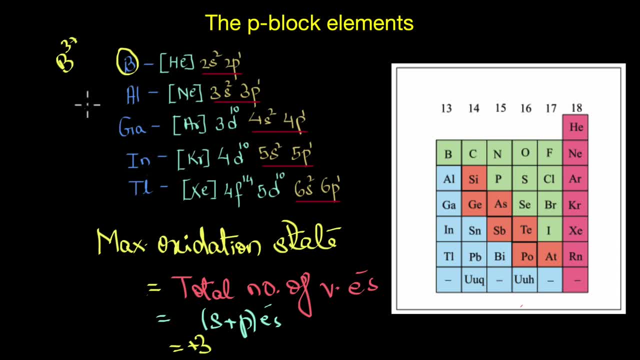 or any other atom forms to be completely ionic in nature and that it attains stability by gaining or losing electrons. all right, now. that's enough recap about oxidation state. now coming back, this maximum oxidation state for a particular group is also called its group oxidation state, and every group has its own specific group oxidation state, depending on. 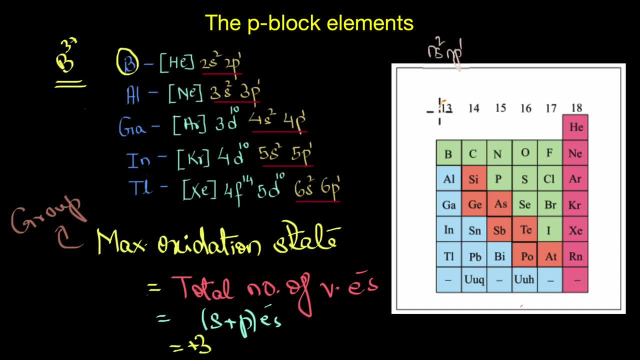 the number of valence electrons, as we just saw, for group 13 it is plus 3. for group 14 it would be plus 4 because it has two electrons in the s orbital and two electrons in the p orbital. for group 15, the group oxidation state would be plus 5 because it has two electrons. 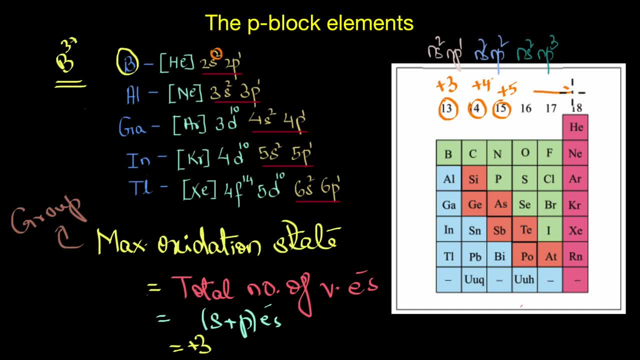 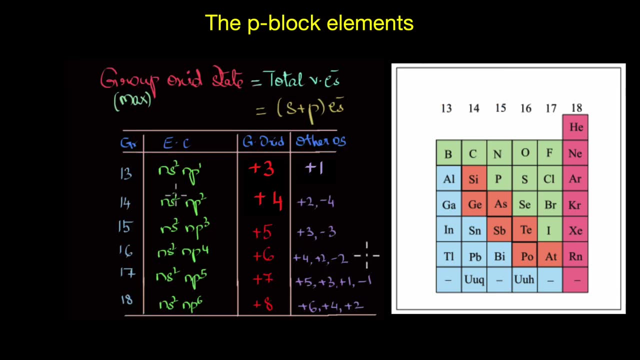 in the s orbital and three electrons in the p orbitals and so on. but you know what? all the elements within a particular group need not have only this particular group oxidation state. in fact, p block elements are known to have multiple oxidation states. for example, in group 13, the 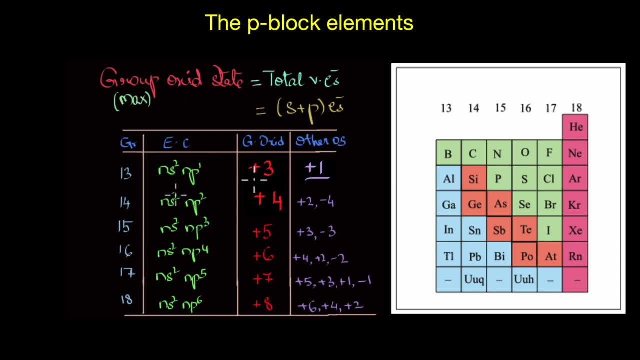 elements show plus one oxidation state in addition to the group oxidation state, which is plus 3.. similarly, in group 14, the elements show plus 2 and minus 4 oxidation states, in addition to the group oxidation state, which is plus 4.. now can you think of a compound. 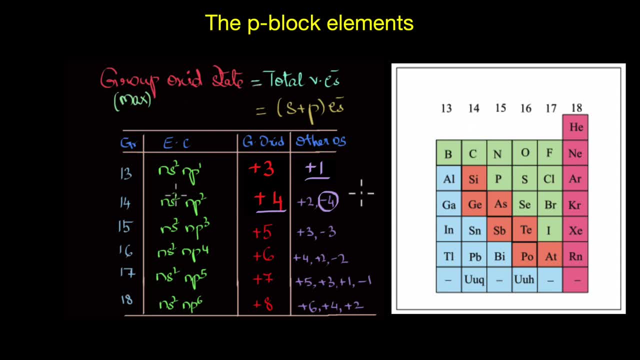 where carbon exists in minus 4 oxidation state. how about ch4? yes, in methane, carbon combines with a more electropositive element like hydrogen, and in this case its oxidation state becomes minus 4, whereas in a compound like co, where it combines with a more electronegative element like oxygen, the oxidation state of carbon 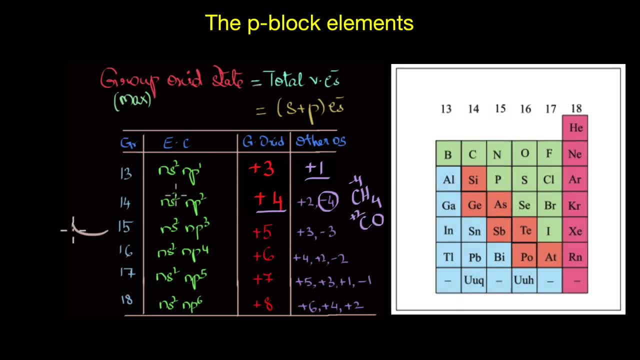 would be a positive plus 2.. now, if you look at group 15, can you name a compound in which nitrogen exists in plus 5 oxidation state? how about nitric acid? yes, in nitric acid nitrogen exists in plus 5 oxidation state, whereas in most amines or ammonia, nitrogen exists in minus 3 oxidation state. 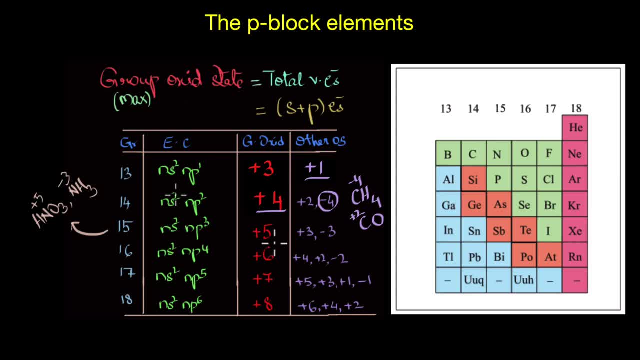 and, just like nitrogen, phosphorus also has many compounds in which it exhibits plus 5, plus 3 as well as minus 3 oxidation states. so basically, as you go across the periodic table or across the p block, the elements tend to show more number of oxidation states. 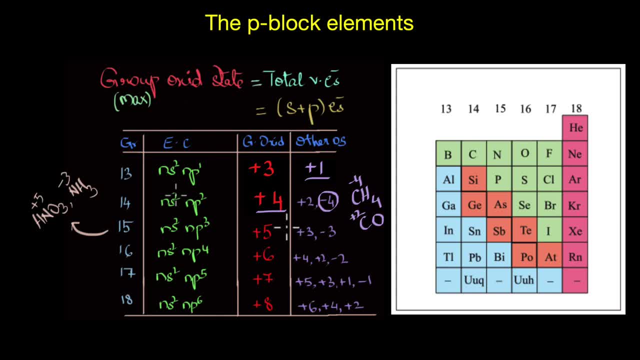 now, in contrast to h block element this is a very significant feature of p block elements, that is, to show variation or variable oxidation states in s block elements. we know that group 1 always shows plus one oxidation state because of group 1, so that is to show that group 1 always. 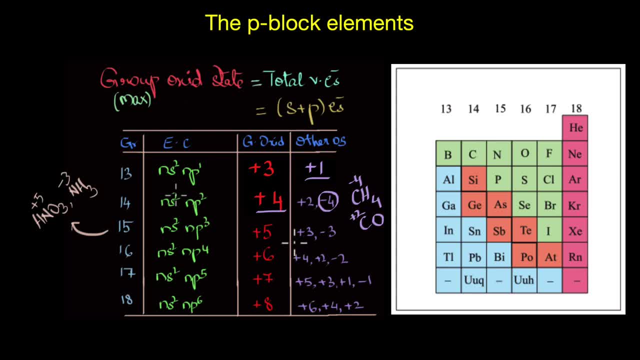 shows plus one oxidation state, whereas group two elements always show plus two oxidation state. but when you come to p block, you will see that the elements tend to exhibit multiple oxidation states. now, before wrapping up this video, i need to bring your attention to something peculiar here. you see, it has been observed that the lighter elements in a group tend 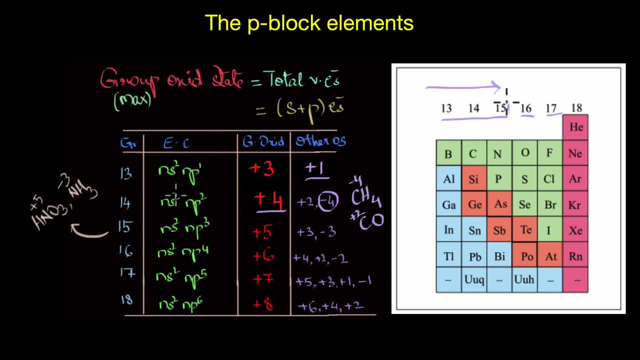 to show the group oxidation state, especially for group 13, 14 and 15, whereas the heavier members within the group become more stable in their lower oxidation state. by lower i mean the oxidation state that is two units lower than the group oxidation state. for example, boron exists only in plus three oxidation state, which is the group oxidation state. but